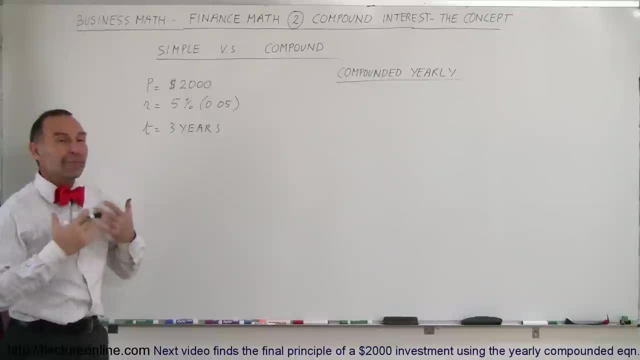 Welcome to our lecture online, and in this video we're going to give you the basic concept of what compounded interest is and the comparison between simple versus compound interest. So here we're working out the problem we did in the previous video. We're investing a principal of $2,000.. We have a 5% interest rate, or 5%. 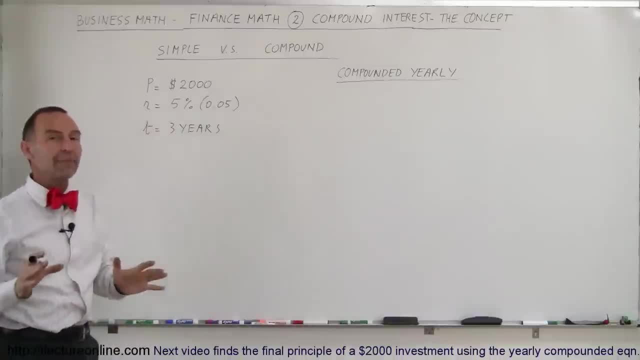 rate, as we call it, and for a time of three years. but it's not compounded, so you only get the interest at the end of three years. So the interest earned is equal to the principal times, the rate times the time. so in this case I would 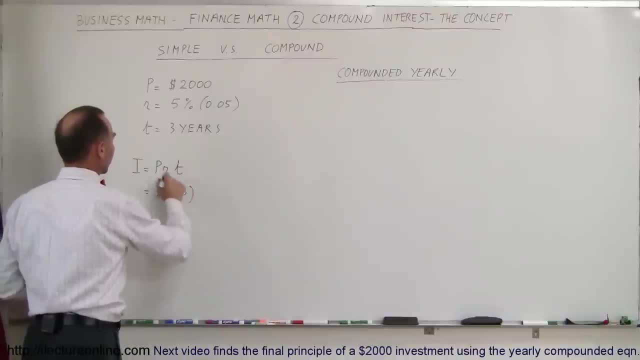 be $2,000 times the rate of 0.05 times the time of three years, and so the total will be six times that. that would be $300.. So that would be the interest earned after three years. but what if they were to compound it? and so we're? 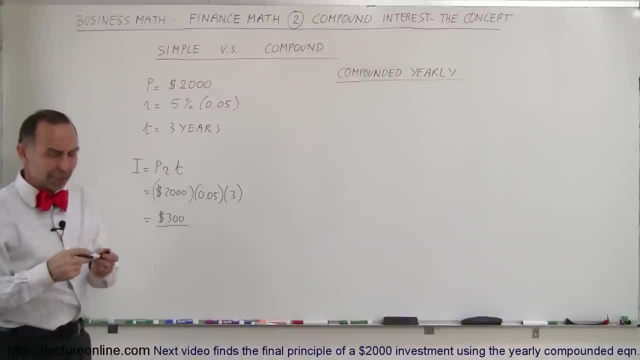 going to start out with a simple concept of compounded yearly. Typically the bank nowadays compounds it daily because we have computers easy to calculate it, easy to compute it. but let's understand the concept. so we're going to start with compounded yearly. That means every year we're going to add. 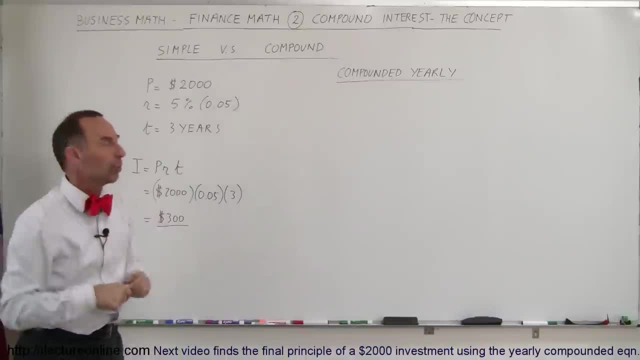 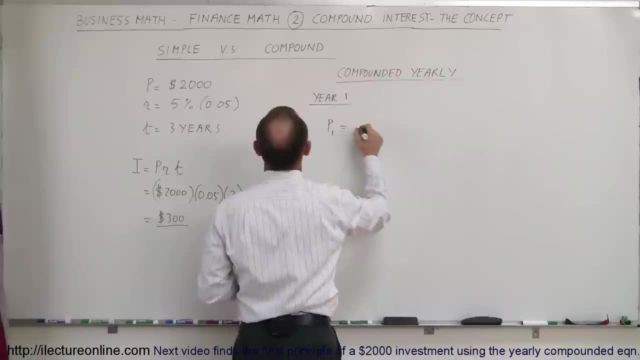 the interest earned to the principal and that will now become your new principal. So year one, the principal earned in after one year is going to be equal to, or I shouldn't say the principal earned for the interest earned to. interest earned after one year is going to be the principal deposited, the first. 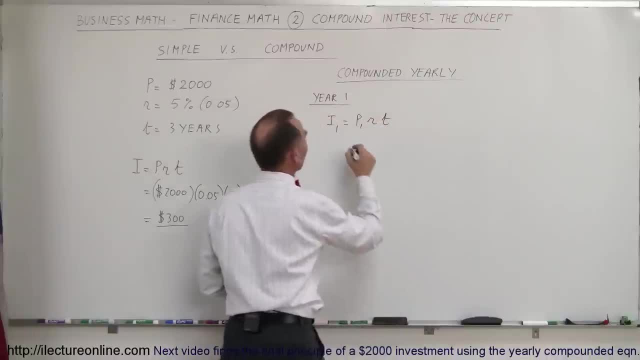 year times the rate, times the time. So in this case that's going to be $2,000 initially invested times the rate, which is 0.05 times the time, which is now just going to be one year, because after one year we're going to add the interest to. 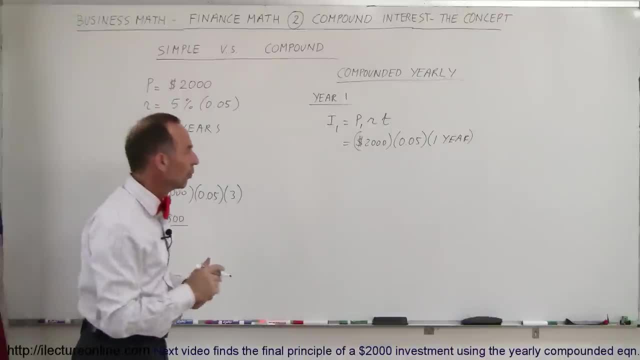 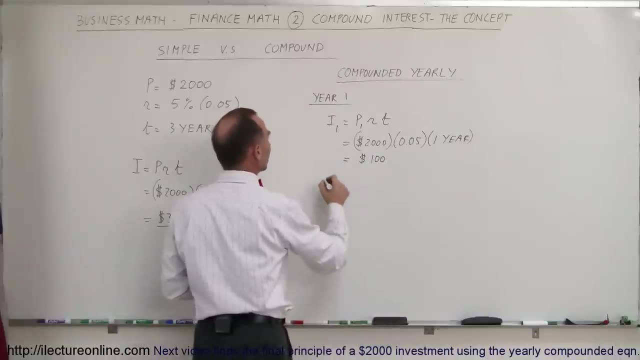 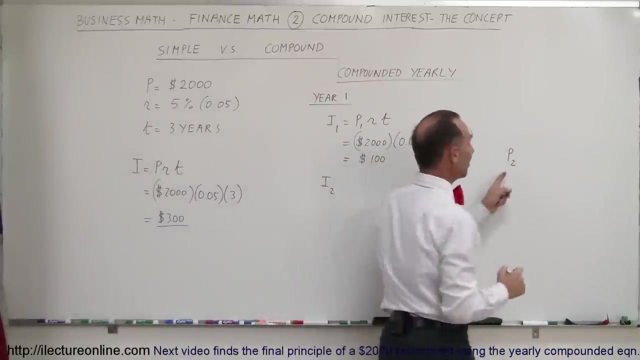 the principal to become the new principal for the second year. So in this case that is going to be equal to $100.. All right, that means that the interest earned in the second year. so, and before I go away, What that means is therefore the principal to be invested in the second. 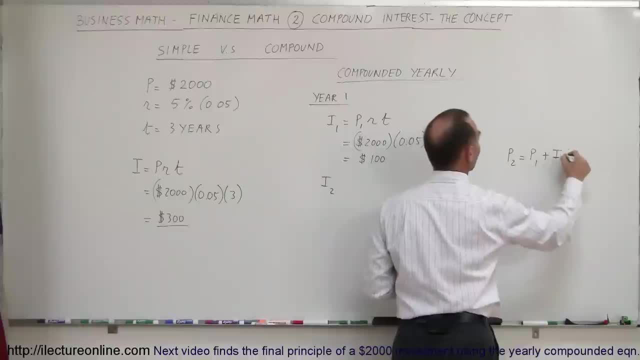 year is going to be equal to the principal in the first year plus the interest earned in the first year. So in this case that's going to be $2,000 plus the $100 that you earned. So now that's going to be an investment of $2,100 for. 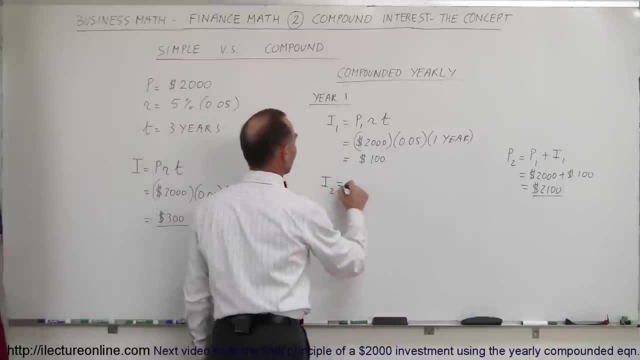 the second year. So the interest earned the second year is going to be equal to the principal of the second year times the rate, times the time. So in this case that's going to be now $2,100.. times the rate of 0.05 times the time of one year. and so this is now going to be. let's see here. 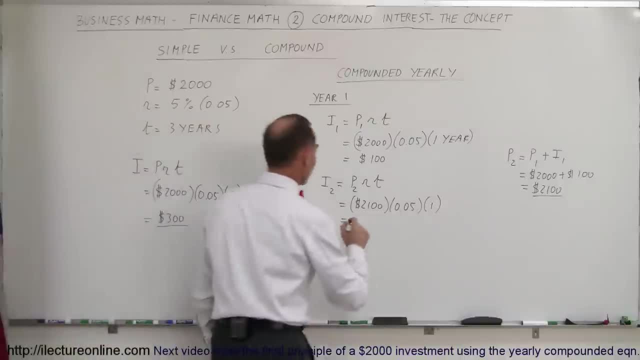 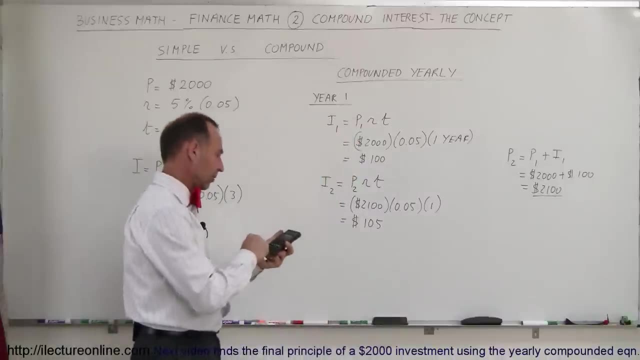 looks like a hundred and five dollars instead. so the interest earned the second year is going to be 105 dollars. well, let me see to make sure i got this correct: 100 times 0.05 and that's 105 dollars. so that is now the interest earned in the second year. so what will now be the principle? that's: 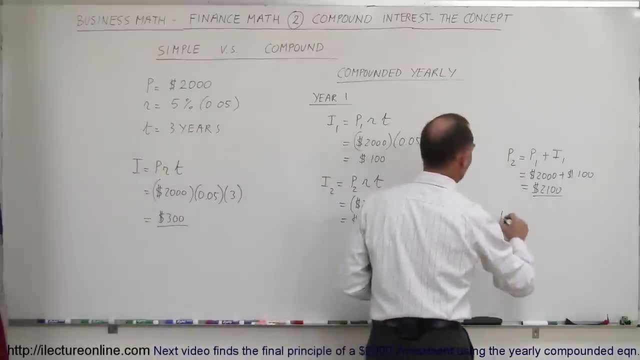 going to be invested in the third year. so you could say now that the principle invested in the third year is equal to the principle invested in the second year plus the interest earned in the second year, which in this case is going to be 200, no 2000, let's see the second year we invested. 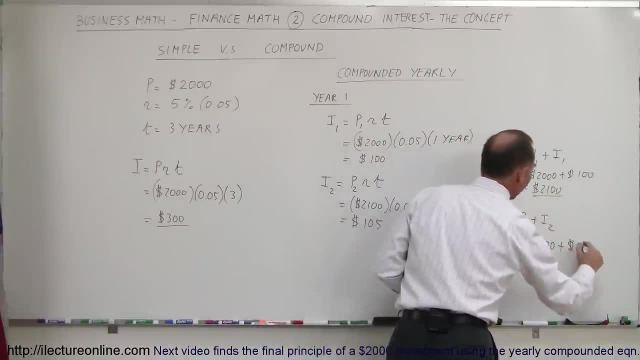 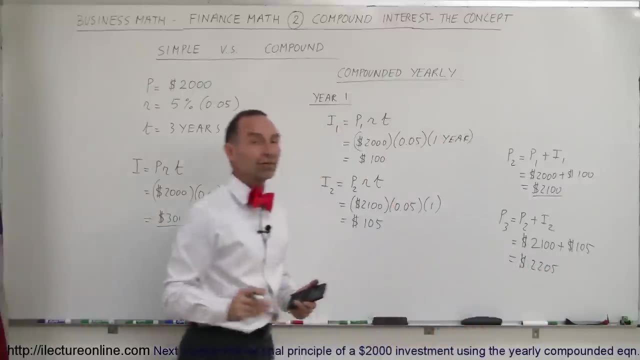 two thousand one hundred dollars and we earned another 105 dollars. so that means we're going to invest two thousand two hundred and five dollars, the third year. that's now going to be the principle for the third year investment. so now the interest earned in the third year is going to be equal to the principle. 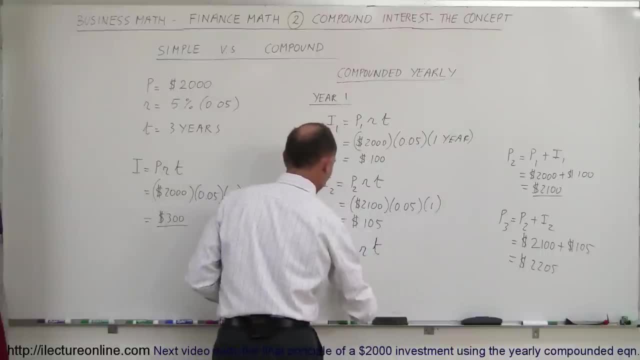 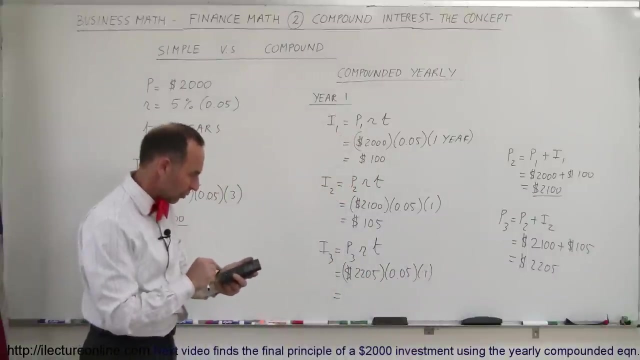 we're investing in the third year. times the rate, times the times. in this case, the principle is now going to be two thousand two hundred and five dollars times the rate, 0.05 times one year. and now let's see what we earn. so that would be 2205 times 0.05 equals. and so now we're going to. 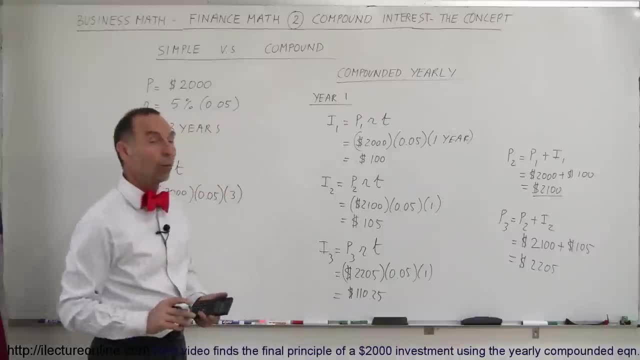 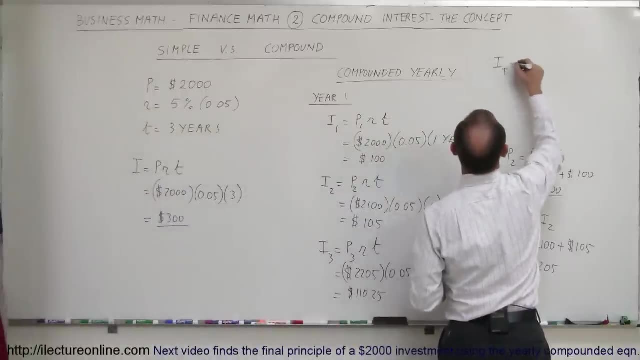 invest two thousand two hundred and five dollars and 25 cents. so what is the total amount of interest that we've earned so we can now write over here? interest total is going to be interest in the first year plus the interest of the second year plus the interest of the third year. so when? 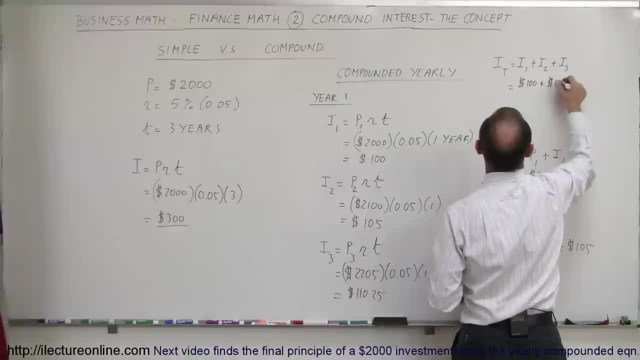 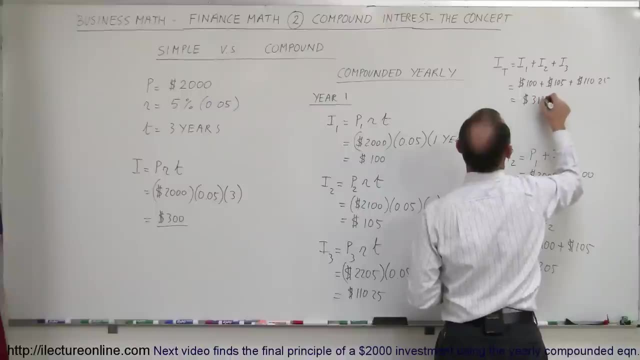 we add them all together, that will be a hundred dollars plus a hundred and five dollars, plus a hundred and ten dollars and 25 cents, for a total of three hundred and fifteen dollars and 25 cents. So how much more money did we earn. how much more interest did we gain.